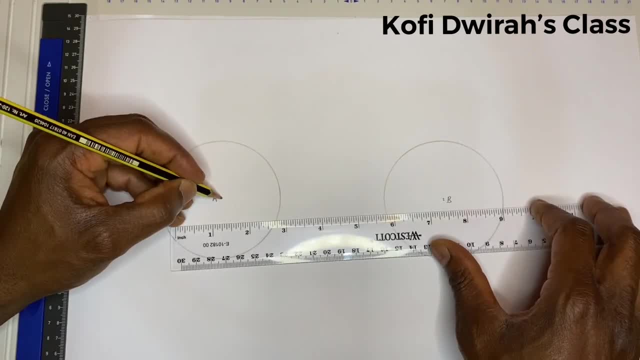 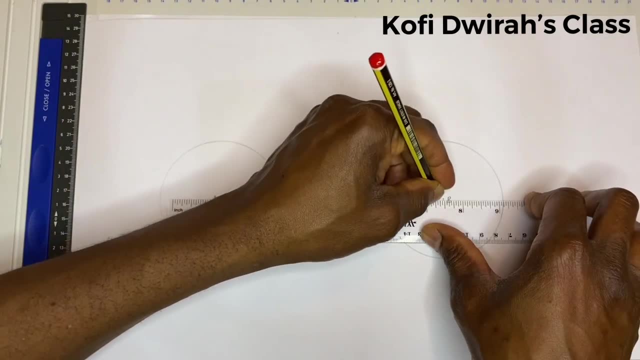 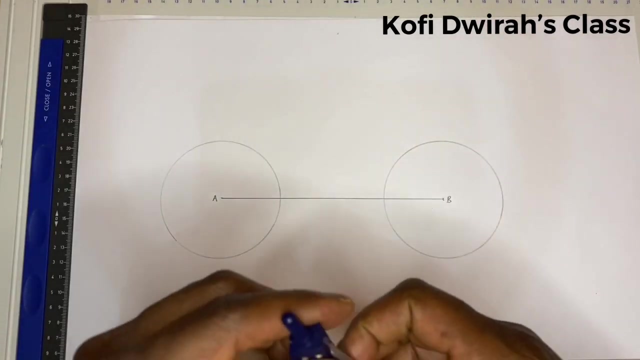 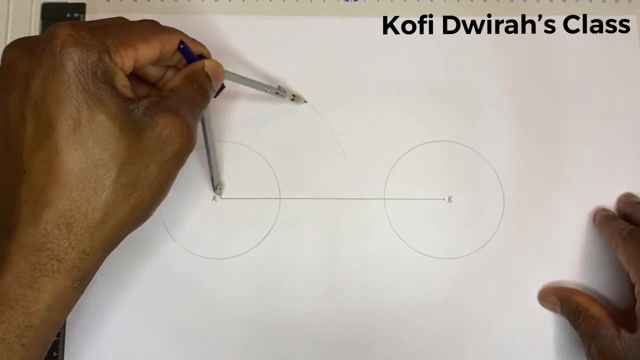 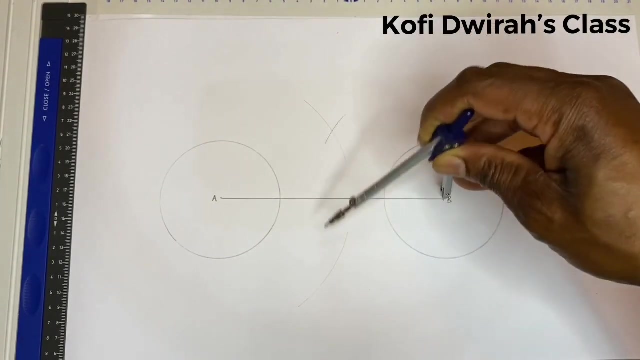 So you draw a straight line From A to B. Good, Then, by set line A B, By set line A B, By set line A B. So at point A you draw your arc, Point B, you draw another arc. 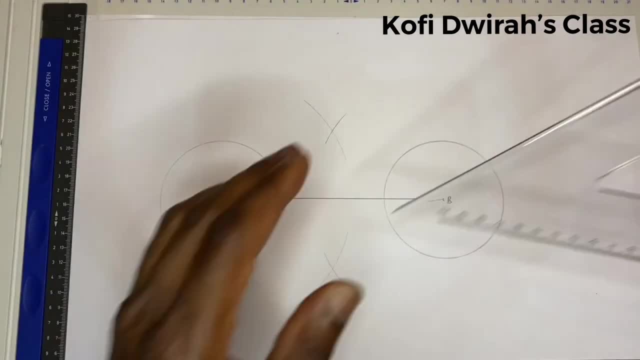 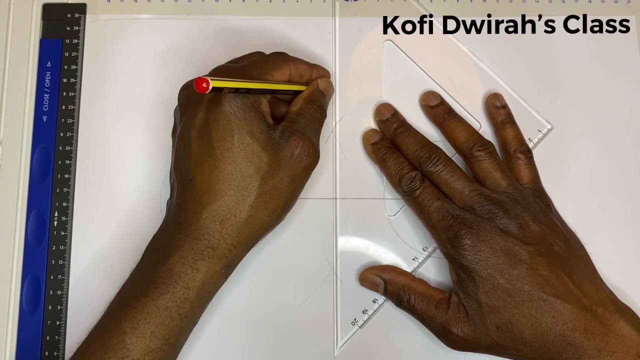 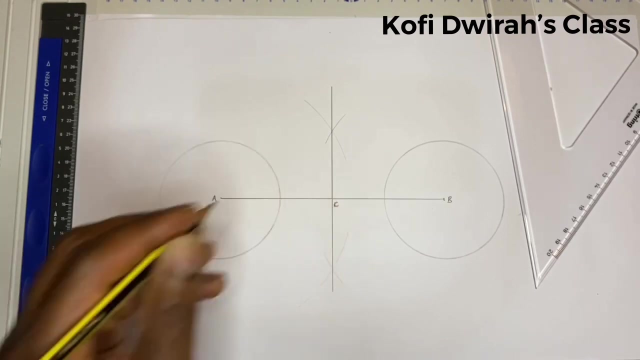 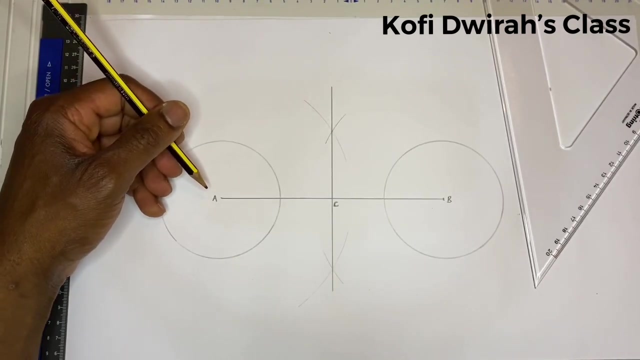 And you draw a straight line. Point B, you draw another arc, Point C: you draw a straight line. Now you have point C, Then by set line A C, Then by set line A C, By set line A C. 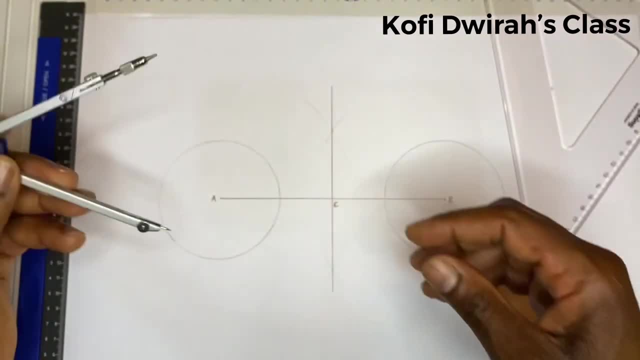 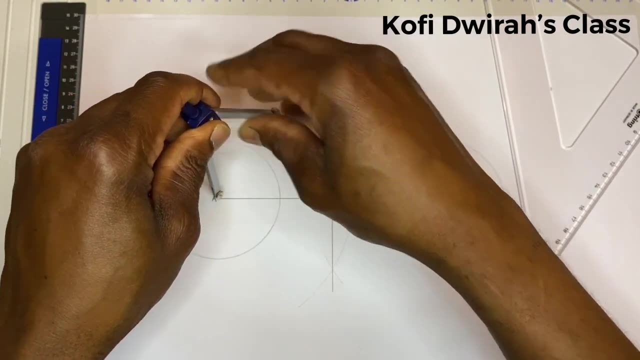 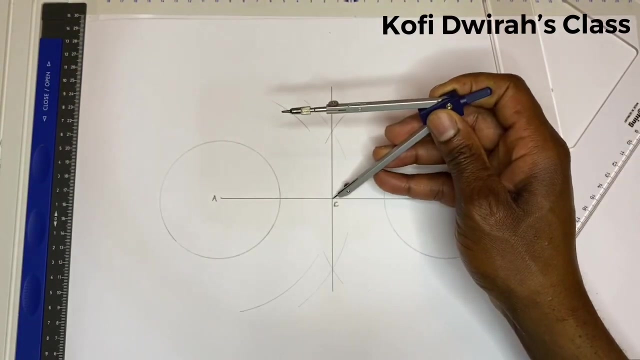 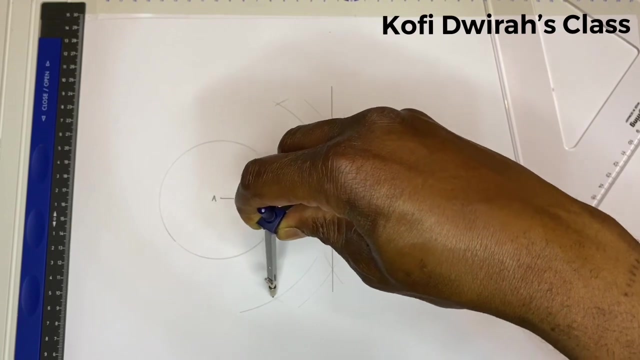 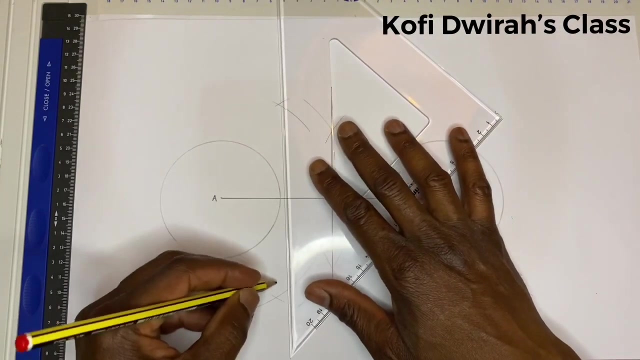 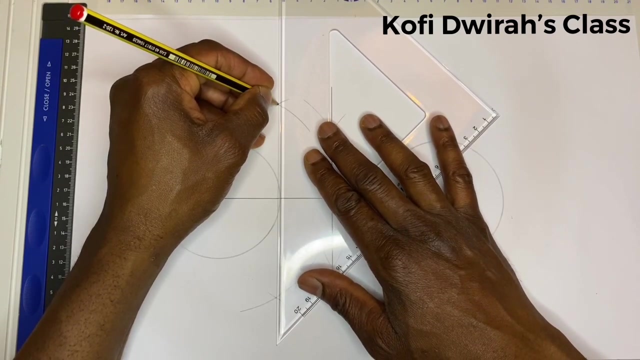 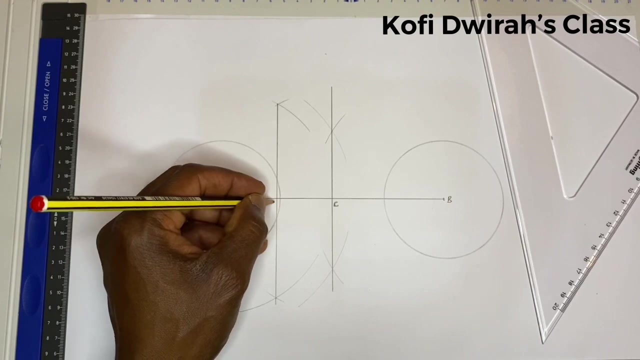 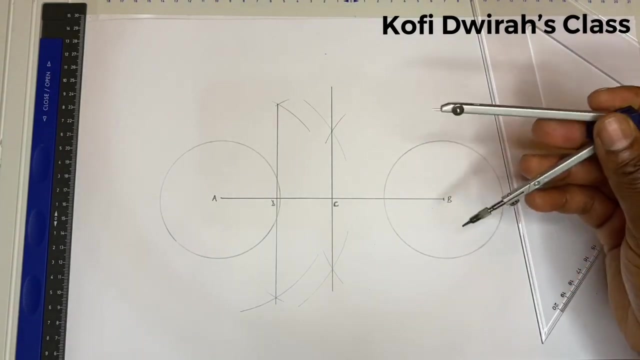 By set line A, C. set like AC, I set like AC. so at point A you draw your arc. at point C, draw another arc and you draw a straight line. draw a straight line. there we have point D, then back to point C. I set like B, C as well. 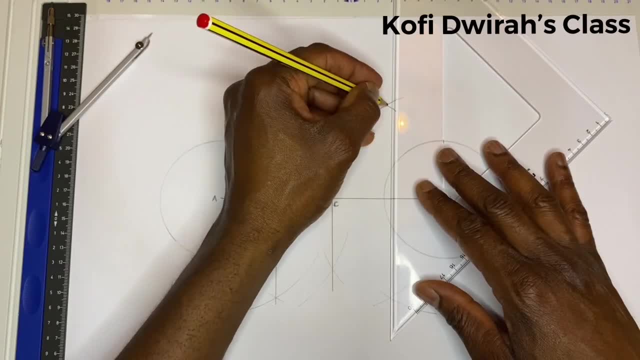 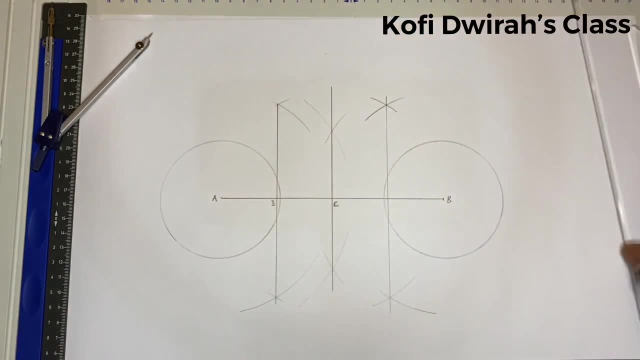 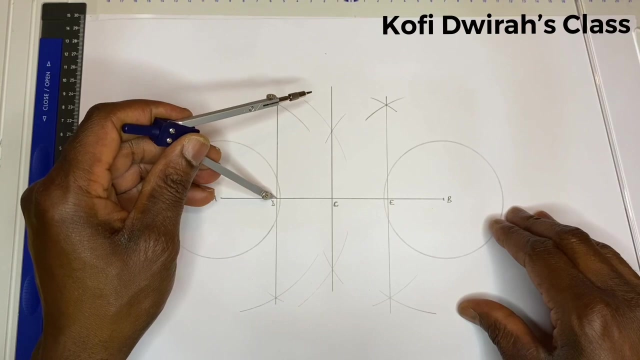 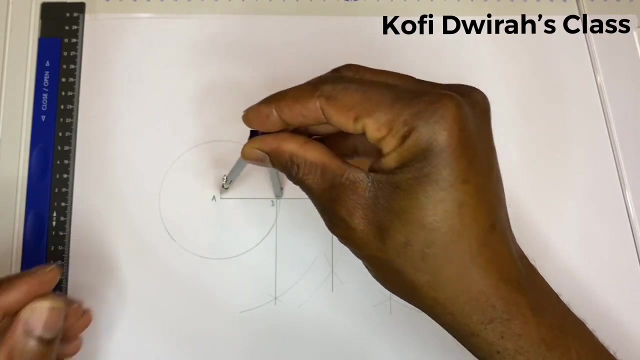 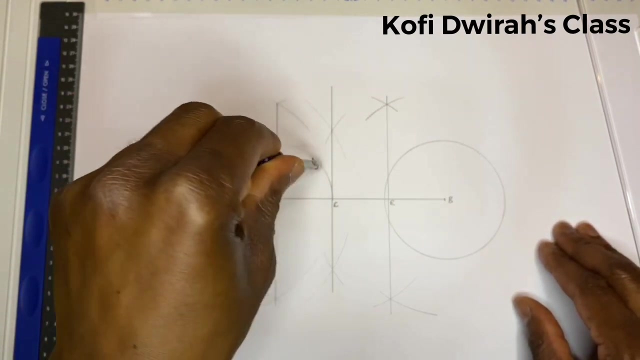 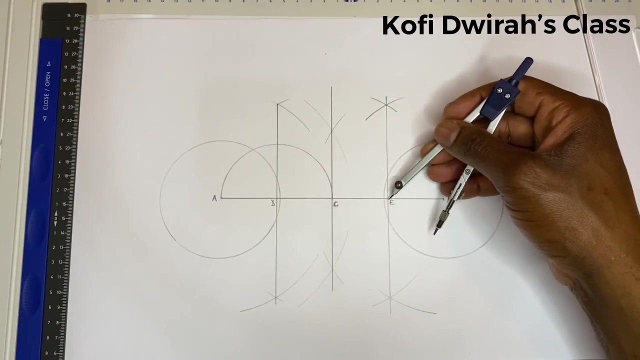 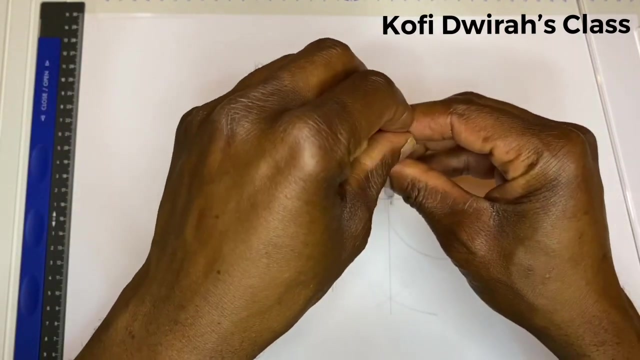 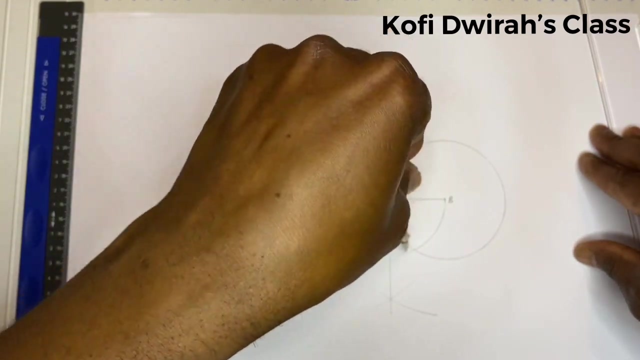 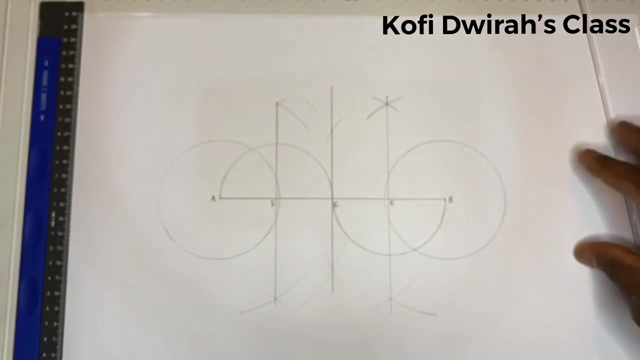 and draw another line, but for to be this point, to be point E, then at point D, when D, you draw a semicircle, draw a semicircle like this, then from point E to C, you draw another semicircle. good, now, this is again like просто. 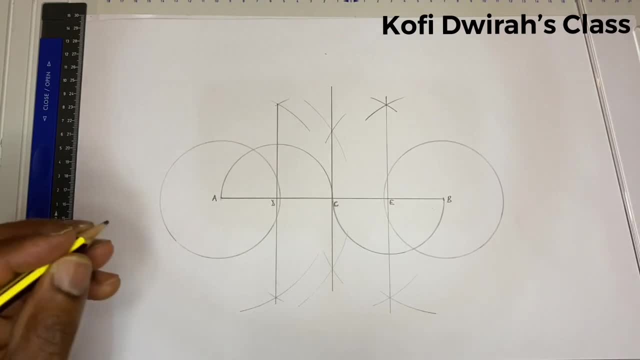 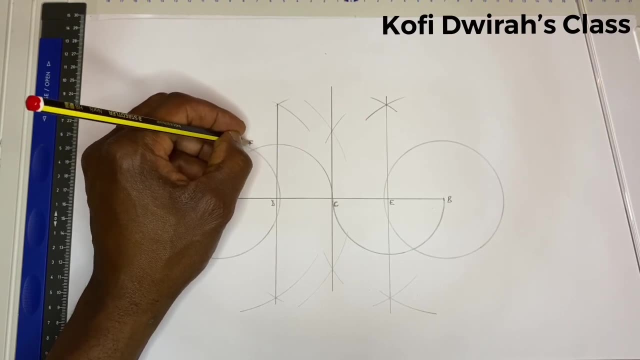 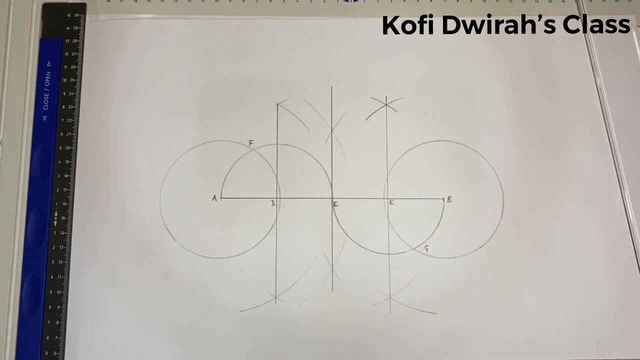 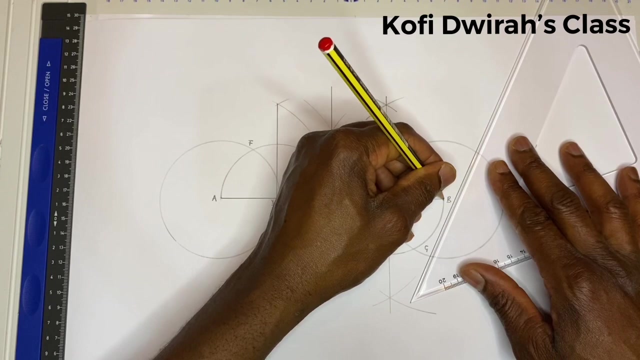 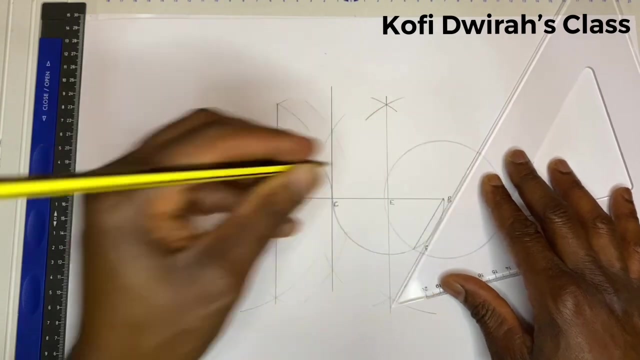 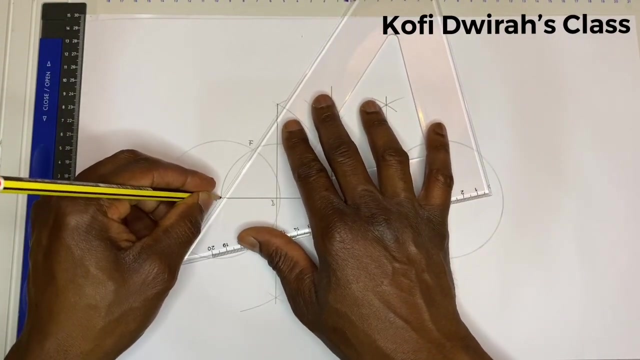 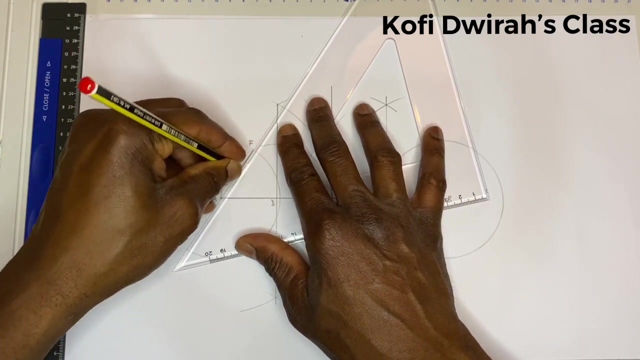 and this is like you draw a straight line. then we have this point to be point F and point G. then draw a straight line from B to left to right and you have bottom point in to the middle, from the bottom point, Jane. so you see it like this. then, from point A to to F, you draw another line. 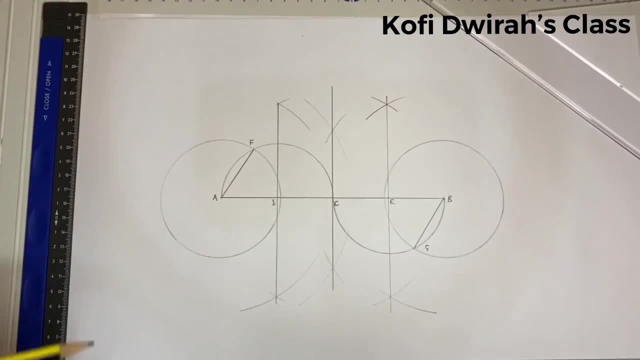 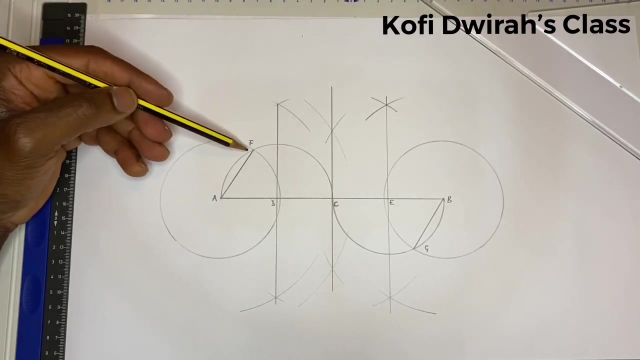 like this. so now we have these lines like E, F and from our one of our lessons, either the path of the circle you know, from here to get the tangent, the angle between the normal and the tangent is always 90 degrees. so this is our normal, so you can extend it a little bit.